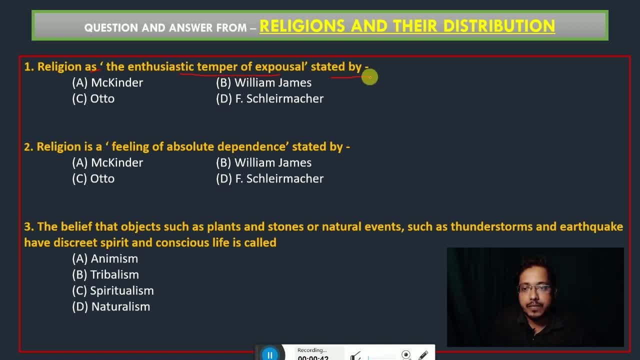 temper of exposure, stated by four options: Option A- Mackinder. Option B- William James. Option C- Otto. Option D, F- Clarimature. The correct answer is option B, William James. Next, question number two: Religion is a feeling of absolute dependence, stated by option A. 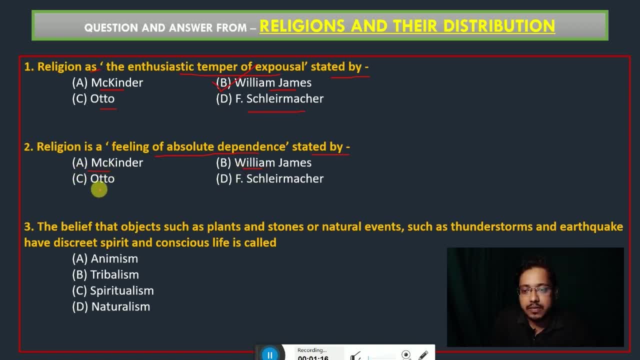 Mackinder. Option D: William James. Option C: Otto. Option D, F- Clarimature. The correct option is Clarimature, So option D is the right answer. Now question number three. They believe that religion is a feeling of absolute dependence, In which religion is. 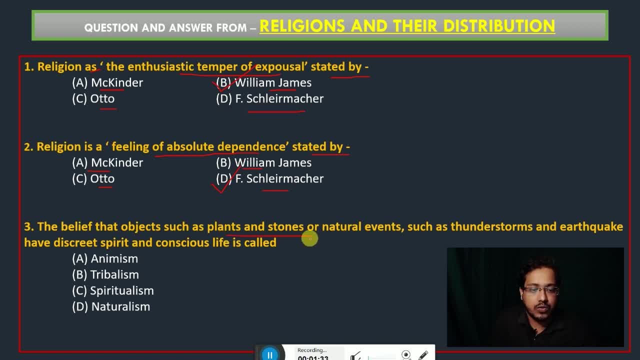 object such as plants and stones, or natural events such as thunderstorm and earthquake, have discrete spirit and conscious life, is called option a- animism. option b- tribalism. option c- spiritualism. option d- naturalism. so here correct answer is animism and how animism is related to this concept. here you see the explanation of the answer. 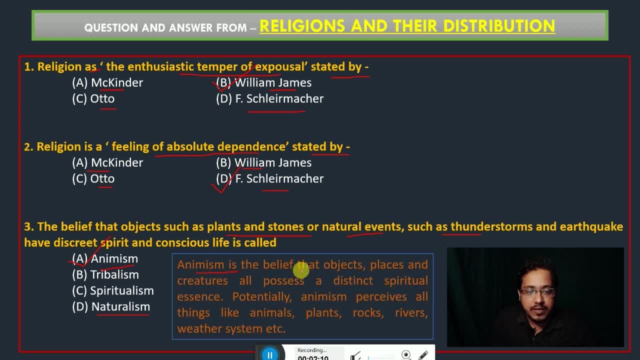 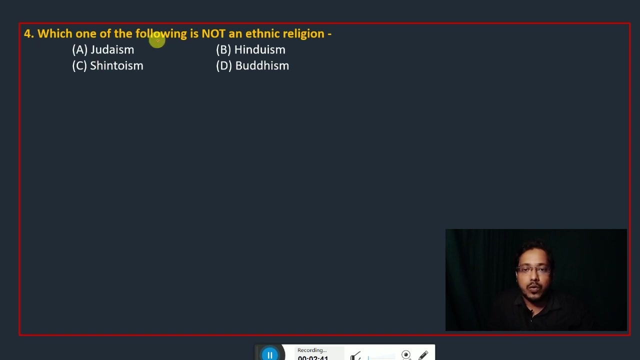 animism is the belief that object, places and creature all possess a district, spiritual essence. potentially, animism perceive all things like en tournament plants, rocks, river, weather system, etc. so correct answer is a animism. question number four: which one of the following is not an ethnic religion? option a- zoodism- option B. Hinduism. option C- Shintoism. option D: Buddhism. so what is not an ethnic religion? so zoodism, Hinduism and Shintoism, these three is ethnic religion and Buddhism is universal religion. so here correct answer is d: buddhism is not an ethnic religion. question number five, which one of the following is not an universal religion: option a: christianity. option b: islam. option c: buddhism. option d: hinduism. so here correct answer is hinduism, because christianity, islam and buddhism, these three are. 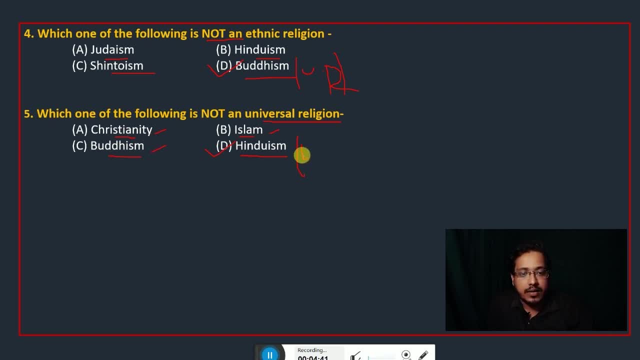 universal religion and hinduism is ethnic religion. so correct answer is hinduism. next question, number six, which one of the following is: a tribal religion has four options: option a- swadism. option b- hinduism. option c- shamanism. option d- buddhism. so swadism and hinduism, these two is ethnic religion. buddhism is. 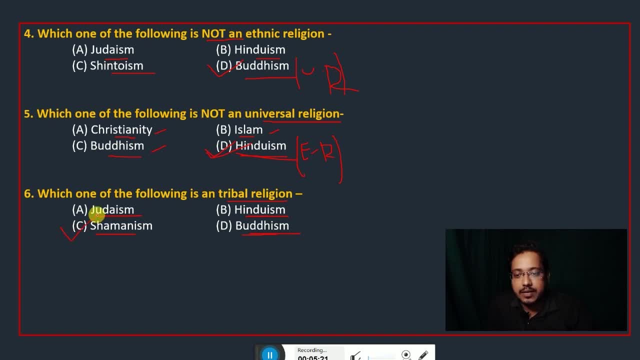 universal religion. so correct answer is c- shamanism. question number seven: the belief of tribal religion is also known as swadism, hinduism, sintoism, animism. so here correct answer is animism, belief of tribal religion. here we see the universal religion and ethnic religion. 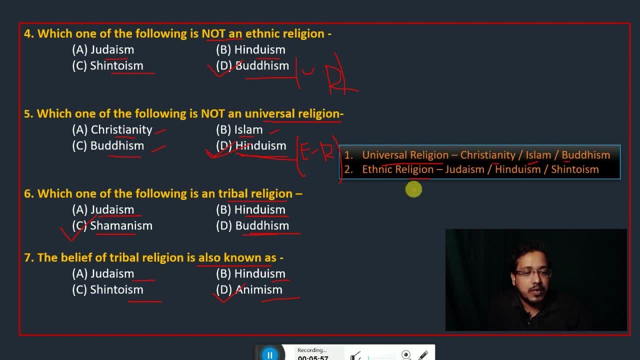 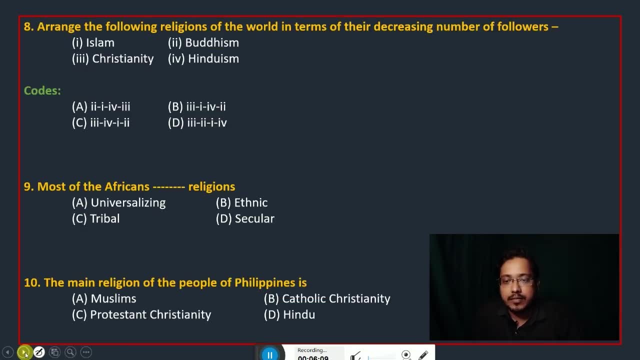 universal religion: christianity, islam, buddhism. ethnic religion, swadism, hinduism, sintoism. question number eight arrange the following religions of the world in terms of their decreasing number of followers: one: islam. b- buddhism. c- christianity. four, hinduism. so what is the correct sequence, in decreasing order? 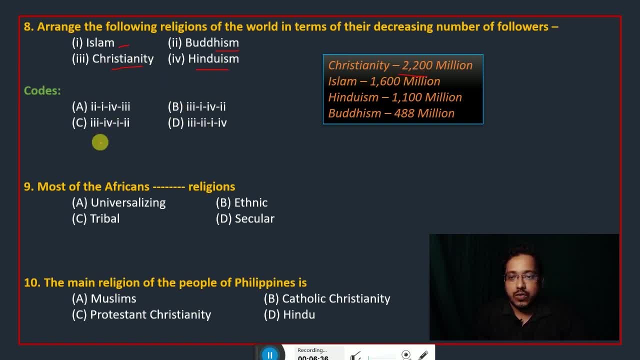 Christianity is the highest, so third, then Islam second highest, so three, one, then hinduism, third highest and then buddhism. so correct sequence is B, three, one, four, two. Next question, number 9.. Most of the African religions- Option A: Universalism, B, Ethnic, C, Tribal, D, Secular. Here correct answer is tribal religion. 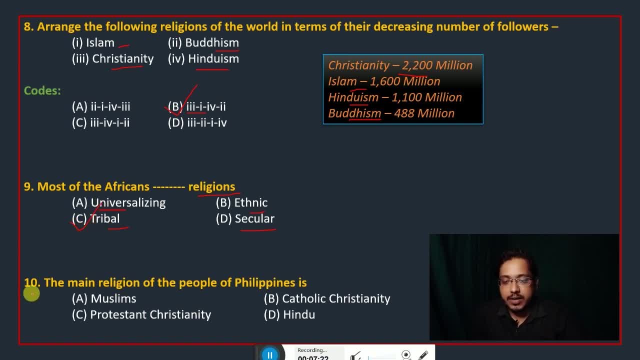 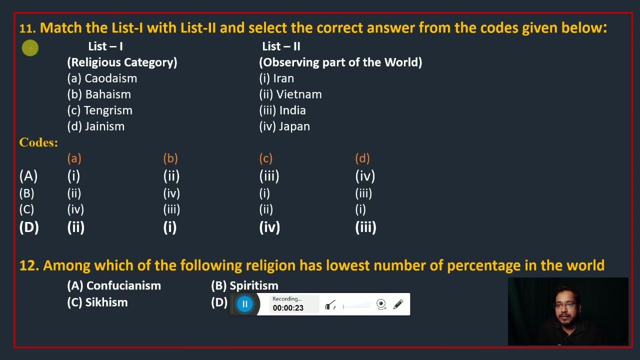 Question number 10.. The main religion of the people of Philippines is, Option A- Muslim, B- Catholic Christianity, C- Protestant Christianity, D- Hindu. So the people of Philippines are from Catholic Christianity. Question number 11.. Match the list 1 with the list 2.. 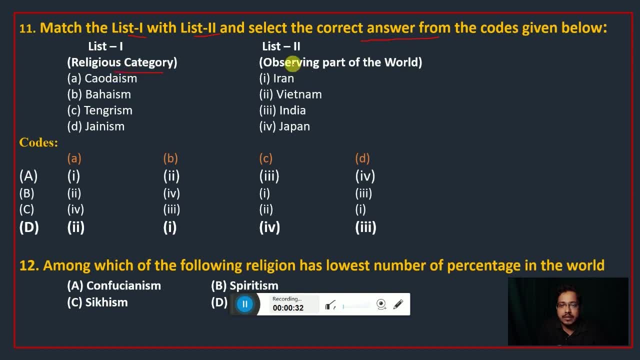 And select the correct answer. So list 1. Religious category And list 2. Observing part of the world. So what kind of religious? A, Quadism, B, Bihism, C, Tengriism, D, Zionism. 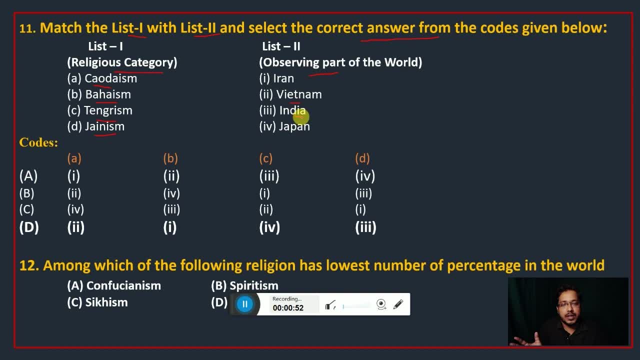 And observing part of the world: Iran, Vietnam, India and Japan. So Quadism A Quadism is from Vietnam, Bihism is from Iran, Tengriism is from Japan And Zionism is from India. So correct answer: A, 2,, B 1,, C, 4, D 3.. So your correct answer is D. Next question number 11.. Question number 12.. Among which of the following religion has lowest number of percentage in the world? 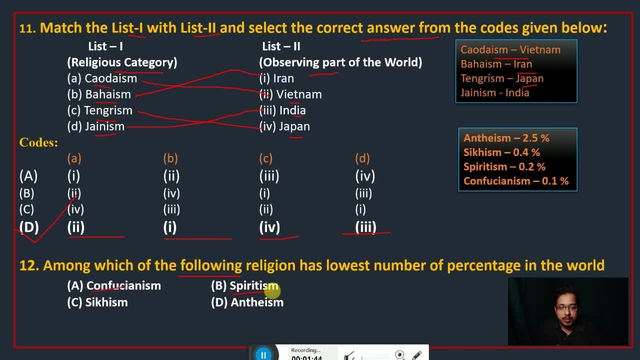 Here option A: Confucianism B, Spiritism C, Sikhism D, Anthism. So here correct answer we see from table: Anthism: 2.5%. Sikh: 0.4%. Spiritism: 0.2%. Confucianism: 0.1%. 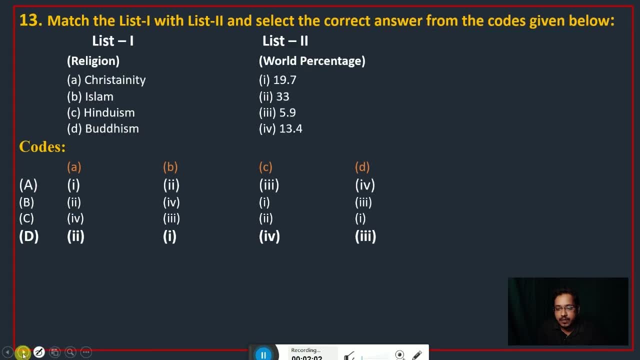 So correct answer is option A, Question number 13.. Match is the least one with least 2. List one: religion category and list 2: court percentage. So religion category: Christianity, Islam, Hinduism, Buddhism. Christianity is highest, which is 33%. 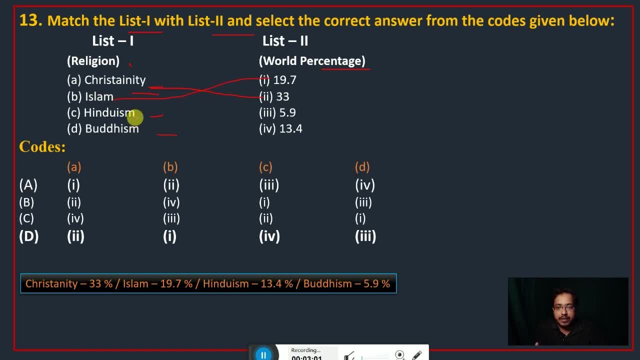 Then Islam 19.7%, Calumni and Abha », aranamma- Greek- Then Hinduism 13.4% and Buddhism 5.9%. So here correct answer is A 2, Islam, B 1,, C 4, D 3.. 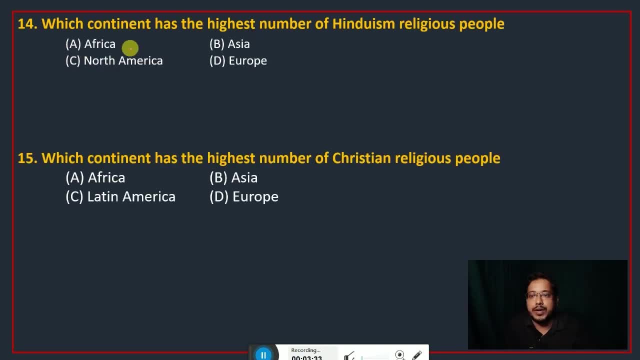 So correct answer is D Question number 14.. Which continent has the highest number of Hinduism and religious people? Which continent? Option A- Africa. Option B- Asia. Option C- North America. Option D- Europe. So what is the correct answer? 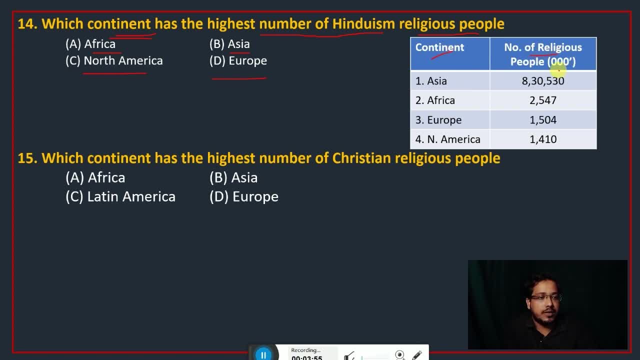 Here you see, with the table, continent and number of religious people in thousand. So number of Hinduism: Asia is the highest: 8,333.. 530 people from Asia. So Hinduism is highest from Asian continent. Next question, number 15.. 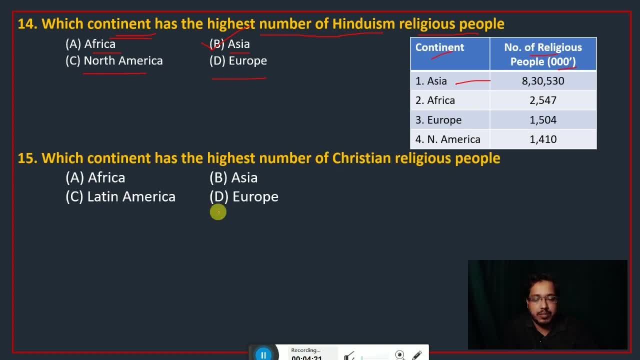 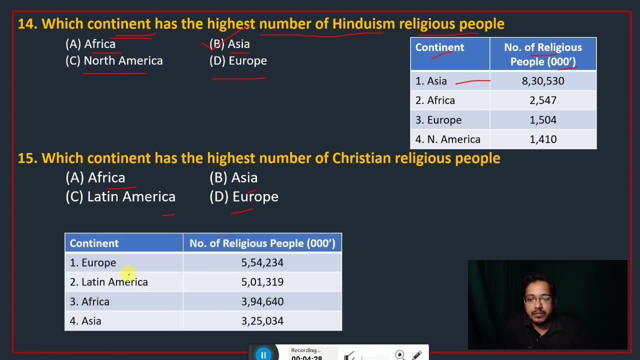 Which continent has the highest number of Christian religious people? Four options: Africa, Asia, Latin America and Europe. So here you see the table. Continent Europe is the highest Christian Religious people: 5,54,234.. So correct answer is Europe. 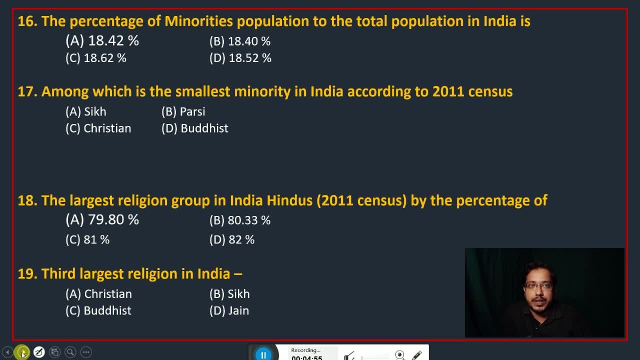 Followed by Latin America, Africa and Asia. Question number 16.. The percentage of minorities population to the total population in India is 18.42%, 18.40%, 18.60% And 18.50%- 18.45%. 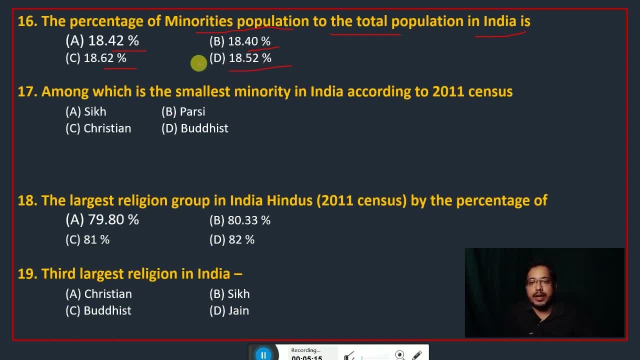 Here, correct answer is the option A: 18.42% among which the smallest minority in India, according to 2011 census. have four options: option A- Sikh. option B- Parsi. option C- Christian. option D- Buddhist. 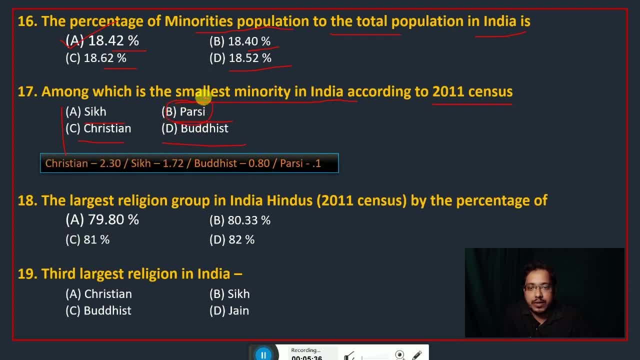 Here, correct answer is Parsi: 0.1%. Okay, Question number 18.. The largest religion group in India- Hindu. according to 2011 census, by the percentage of option A: 79.80%. option B: 80.33%. option C: 81%. option D: 82%. 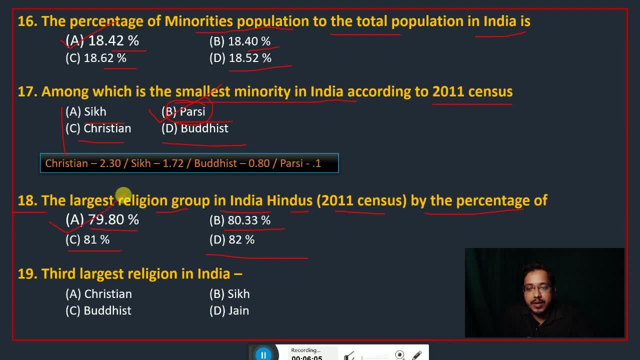 Here, the correct answer is 79.80%, according to 2011 census. Question Question 9.. Third largest religion in India- option A- Christian. option B- Sikh. option C- Buddhist. option D- Jain. Third largest religion group in India is Christian. 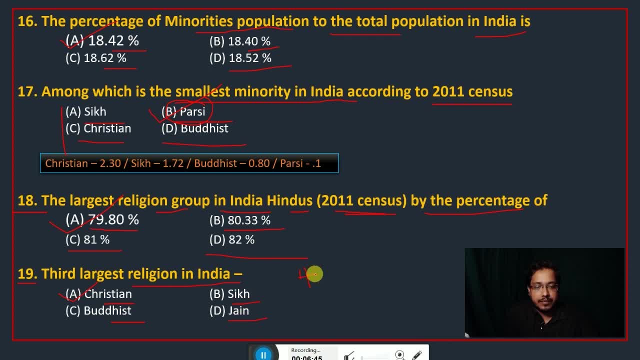 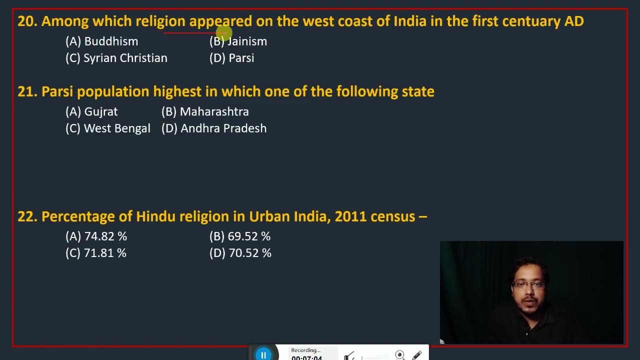 First Hinduism, Second Islam And third Christianity. So correct answer is Christian. Question number 20.. Among which religion appeared on the west coast of India in the first century? AD? Option A: Buddhism. option B: Jainism. option C: Siren Christian. option D: Parsi. 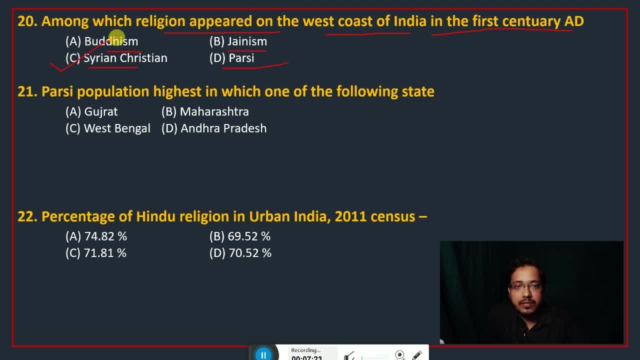 Here. correct answer is Siren Christian, which is appeared in Indian west coast in the first century AD, Question number 20.. The Parsi population is highest in which of the following states: Option A: Westeros, Western Bengal and Indian West Bengal. 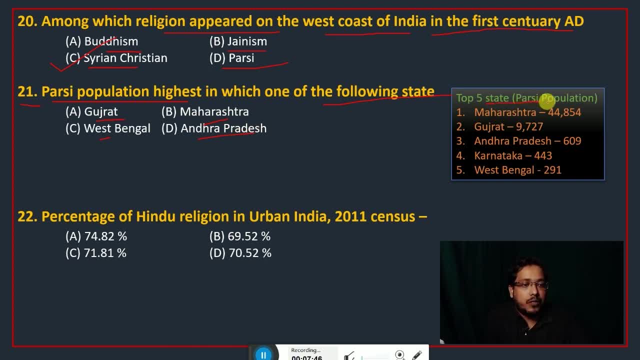 Here you see the table of top five state Parsi population in India And the top is Maharashtra, which is 44,854.. Followed by Gujarat, Andhra Pradesh, Karnataka and West Bengal, Question 9.. so here is the correct answer: is Maharashtra. option B. question number 22. 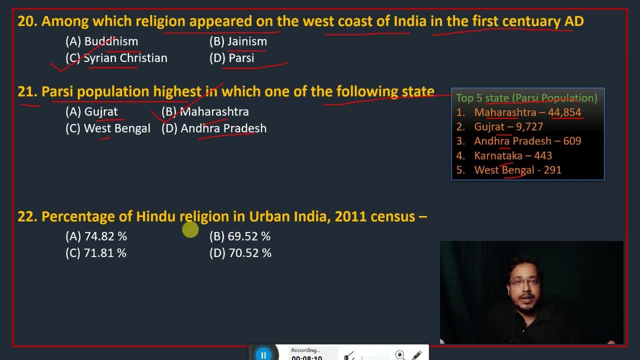 percentage of Hindi religion in urban India according to 2011 census: option A: 74.82. option B: 69.52. option C: 71.81. option D: 70.52%. so correct answer is urban Hindu: 74.82%. so correct answer is A you also. 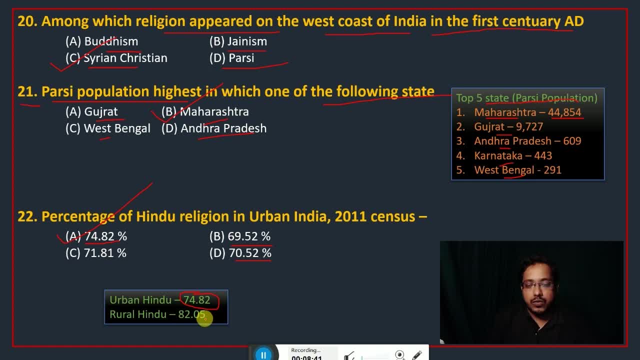 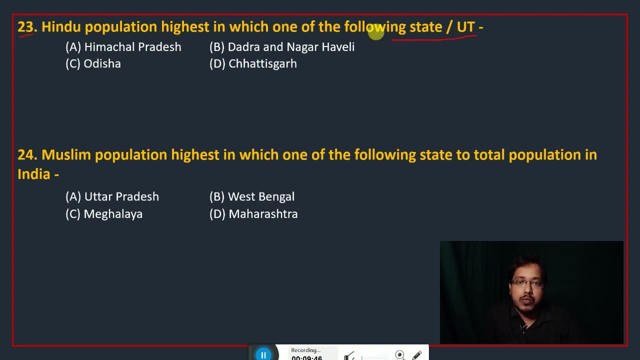 remember %the percentage of rural Hindu. so what% of rural Hindu? 82.05%? question number 23: Hindu population highest in which of the following state or UT: option A- Himachal Pradesh. option B- Dadhra, opposion ble. option C- Kurdish. on reason C. 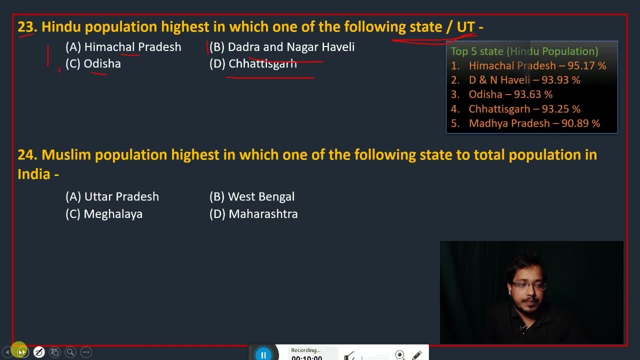 option one, exception B. so here you see the table top five: state or ut hindu population: first in himachal kodesh regarding state and first dadra nagar haveli regarding union territories. so here is the correct answer: is himachal kodesh. 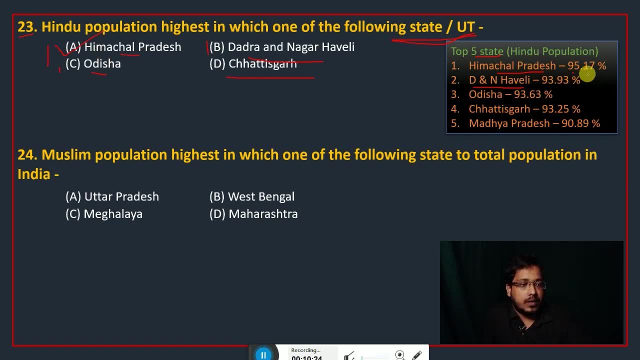 95.17 percent. question number 24: muslim population highest in which of the following state to total population in india. so what is the correct answer? option a: uttar potash. option b- us bengal. option c- meghalaya. option d- maharashtra. so her top five state? 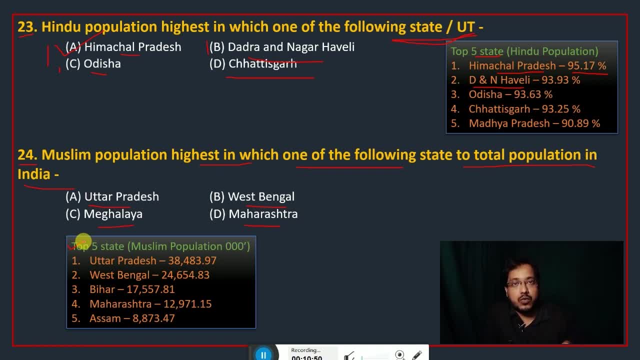 muslim population regarding total population in india. so to the total population of india, muslim population highest in uttar potash, followed by west bengal, bihar, maharashtra and assam. so her correct answer is: uttar potash population is 38 483. all the population are in thousand. figure question number 25: percentage of muslim. 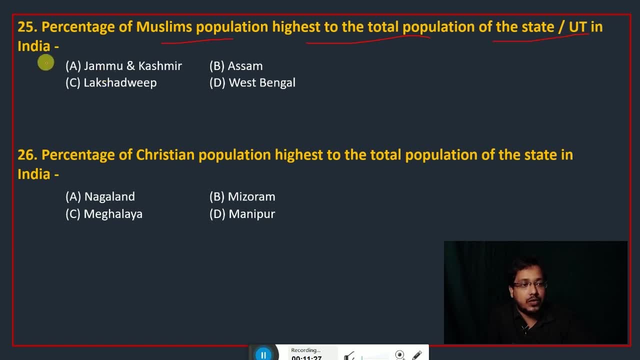 population highest to the total population of the state of india. ut in india. option a: jumbo, kashmir. option b: assam. option c: lakha. option d: west bengal. so here you see the table: lakha, 96.58, then jumbo and kashmir 68.31. 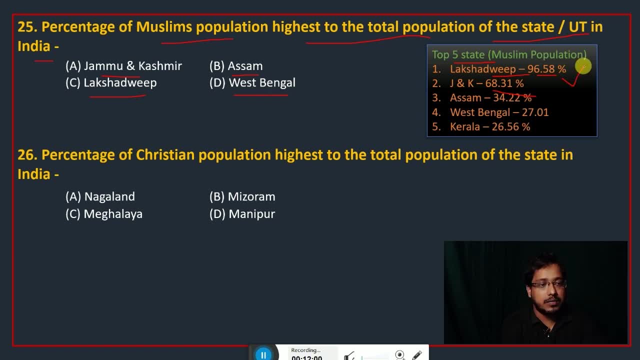 so, regarding ut, lakha diva is the highest and regarding state, jumbo and kashmir is highest. so here is the correct answer: is lakha diva because of state and ut also noted here. so here is the correct answer: is lakha diva 96.58. 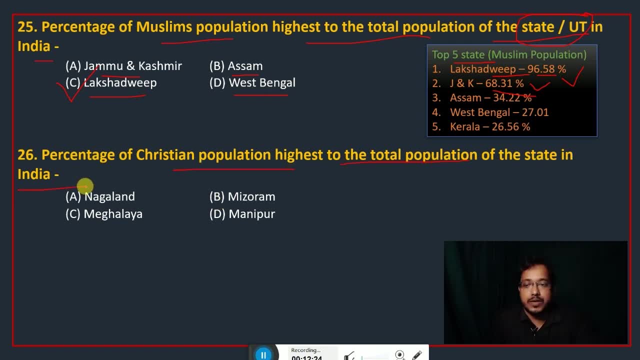 percentage of christian population highest to the total population of the state in india. question number 26: option a, nagaland. option b, mizoram. option c, meghalaya. option d, manipur. so so here top five. state of christian population: nagaland: 87.93 percent. so her correct answer is a.